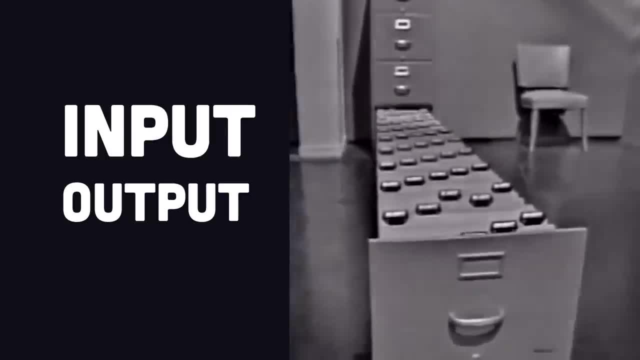 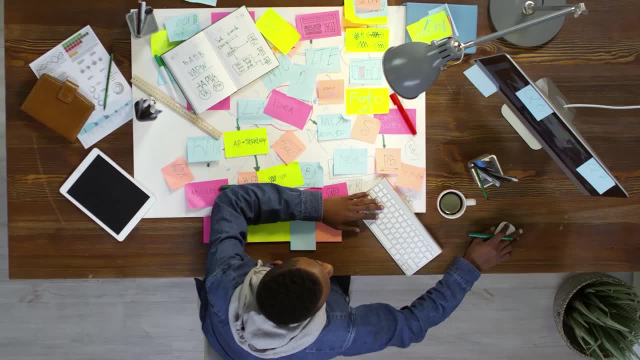 work like reading and writing to a database, the file system or network communication, Because in those cases you're waiting for the disk or the network to supply the actual data and the CPU can't do a whole lot to speed that up, So it's important to keep in. 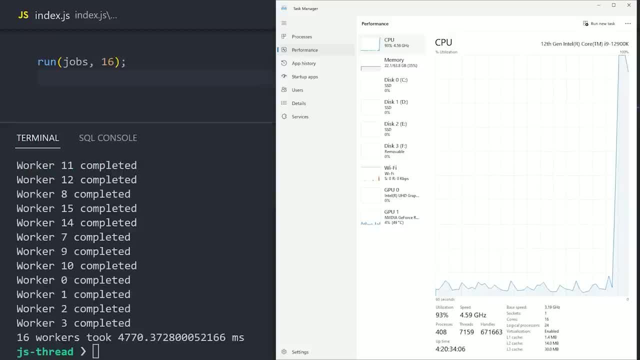 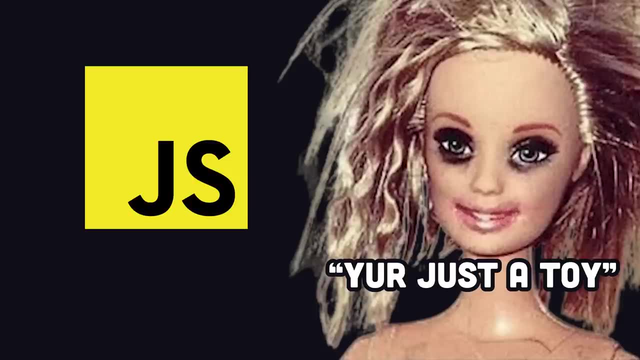 mind that multi-threading doesn't just magically speed everything up. It's just a way to distribute work across multiple CPU cores when the CPU is doing the heavy lifting. Historically, people have criticized JavaScript as a toy language, in part because it was. 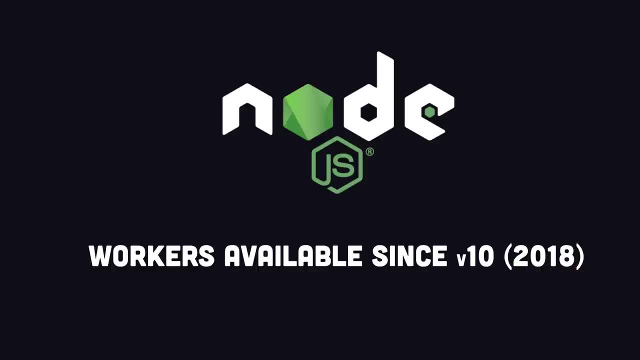 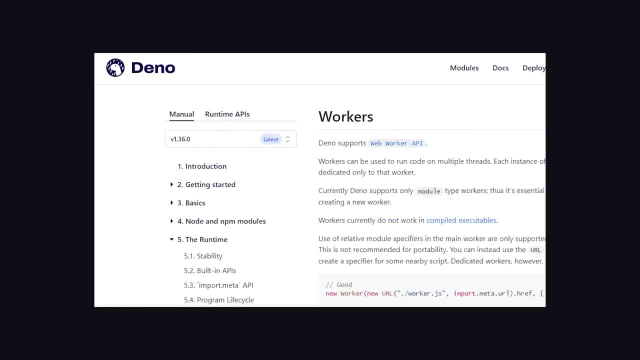 single-threaded, but it's actually been capable of multi-threading for many years. There are libraries like PartyTown that use WebWorkers to run scripts in the background, and that same API is also supported in Deno. but what we're going to look at today is the Workers. 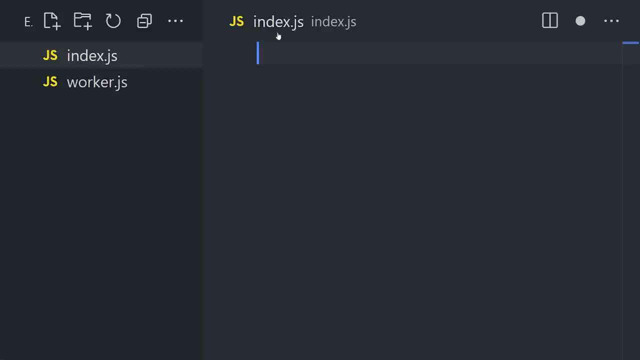 API in Nodejs To follow along, simply create an indexjs file in your editor. Now, before we get into Workers, I first want to simulate a CPU-intensive task that would block the main thread. Let's imagine we have an array of jobs to simulate something that we 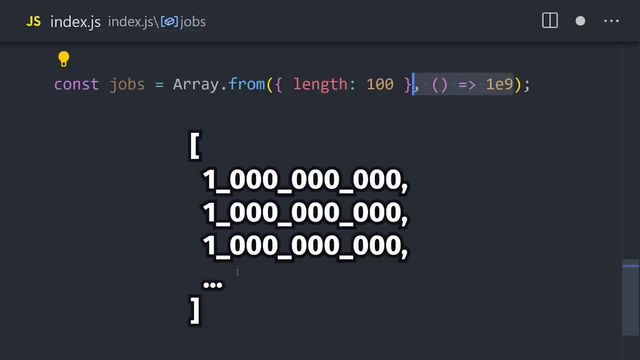 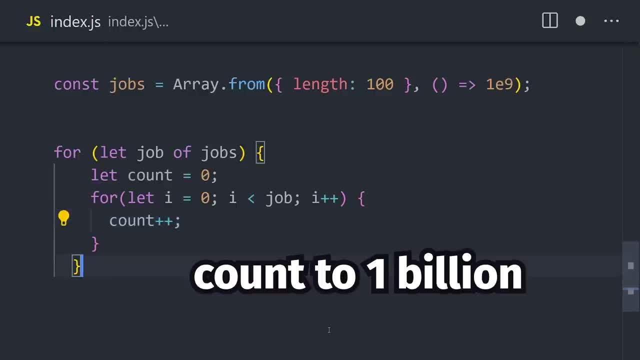 need to compute. In this case, I'll just populate that array with the number 1 billion, 100 times. From there we'll create a nested for loop that loops over each one of those jobs, then simply iterates from 0 to 1 billion until it reaches the end. Totally pointless, but 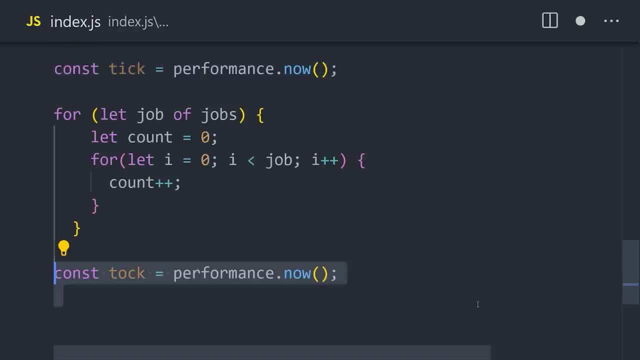 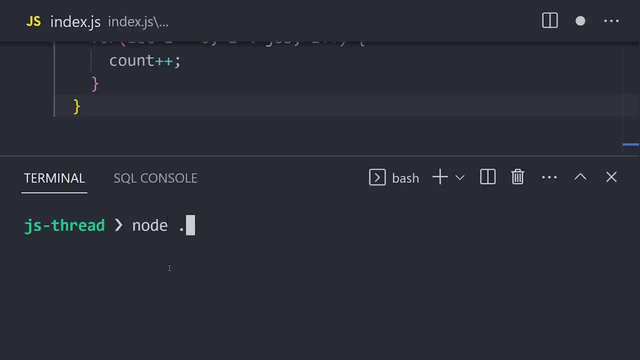 it's good exercise for the CPU. Now let's go ahead and use the performance module to grab a timestamp before and after this code runs to measure the execution time. Now we can go ahead and open up the terminal, run the Node command and wait. In my case it. 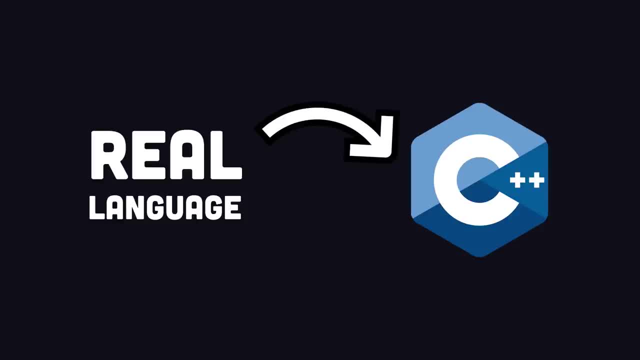 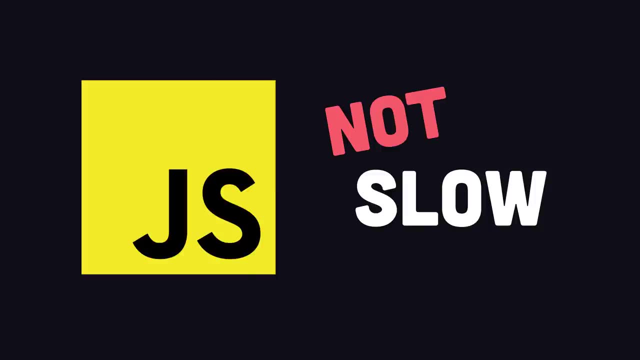 takes seconds to count to 100 billion. That's a lot faster than I could do it, but not very impressive compared to a compiled language running on multiple threads. However, contrary to popular belief, JavaScript is not slow When it's just-in-time compiled by V8, it. 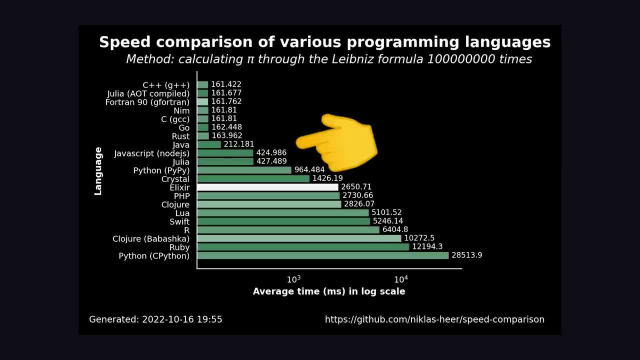 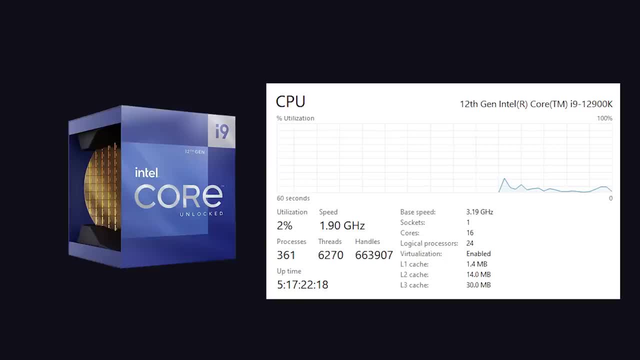 actually performs way better than many other interpreted languages, because V8,, which is built with C++, compiles it to machine code before executing it. Performance will vary based on your machine and in my case I have an Intel i9 processor with 8 physical cores. 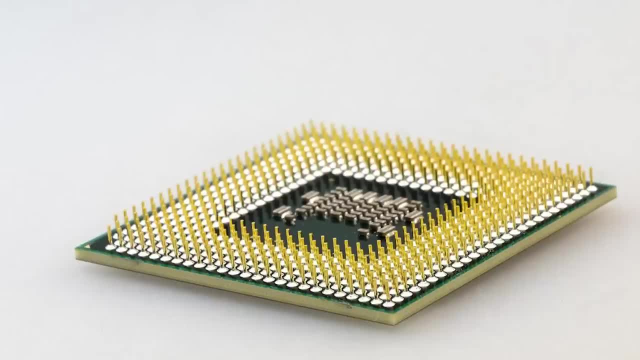 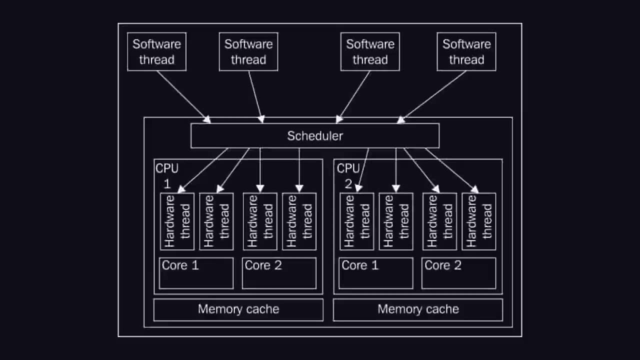 but because it does hyperthreading, we technically have 16 cores to work with. Just a side note: a core refers to the physical component of the CPU itself, which can only execute one task at a time, whereas a thread refers to a sequence of instructions that can be managed. 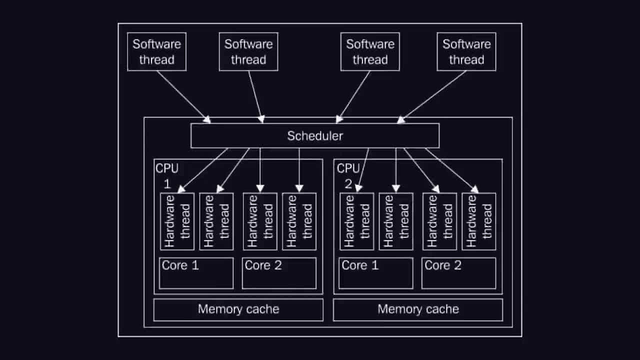 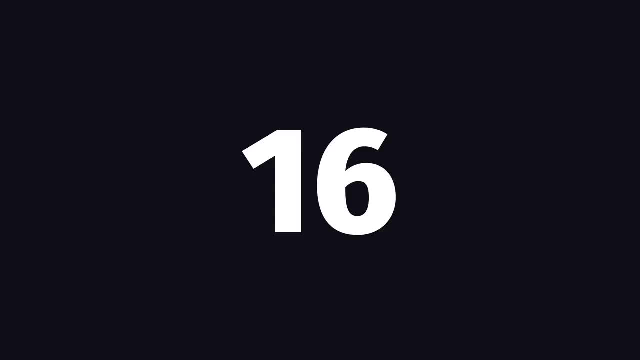 independently by the operating system's scheduler. There's a distinction to be made there. but from a practical standpoint, the amount of Nodejs workers you can run in parallel is equal to the available number of CPU cores, which in this case is 16.. Now to keep this. 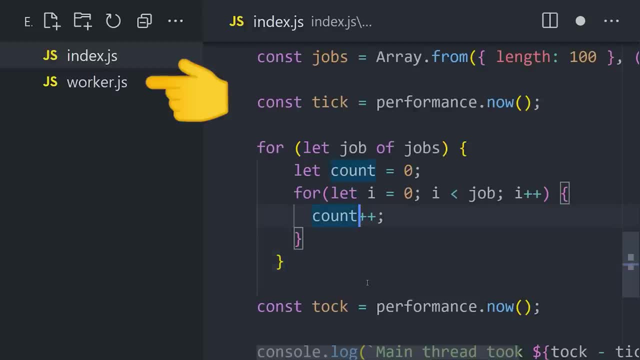 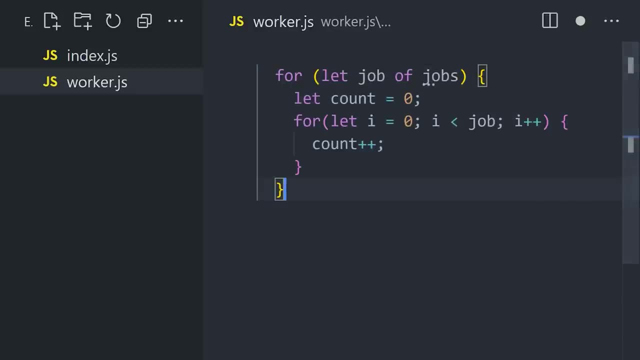 code organized. I'm first going to create a new file called workerjs, and we can simply move the loop that does the actual work into it. The goal is to have the code in this file, not run on the main thread. We could actually combine all this code in a single file, as the node worker module allows. 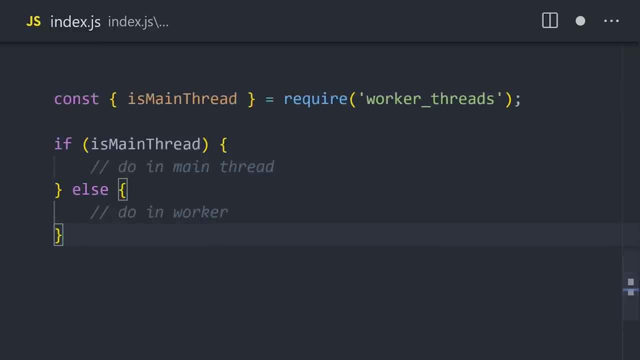 you to check if you're actually on the main thread. but I think it's a lot easier to reason about when you put your worker in a separate file And back in the main file. I'll go ahead and import the worker class from the worker threads module. Then from there I'll create. 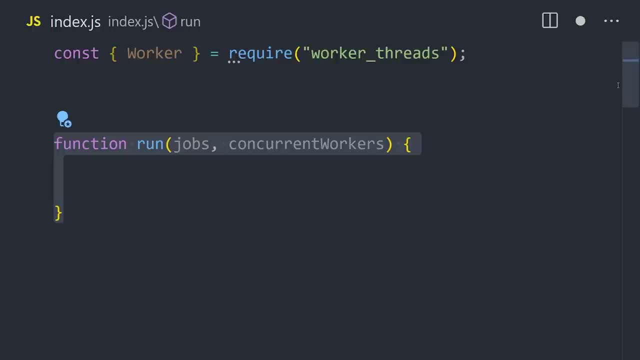 a function that takes the array of jobs as an argument and then also specify the number of concurrent workers or threads that we want to run in parallel. From there, I defined a helper function called chunkify that will take the initial array of jobs and then split. 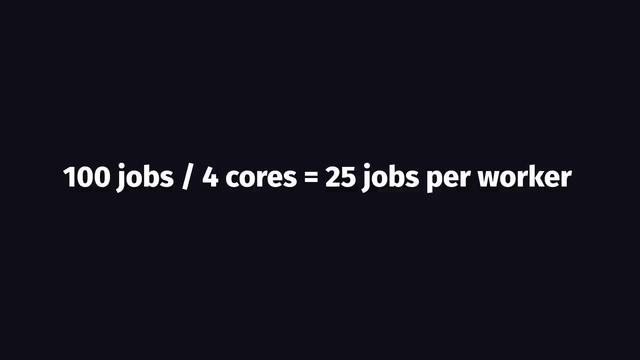 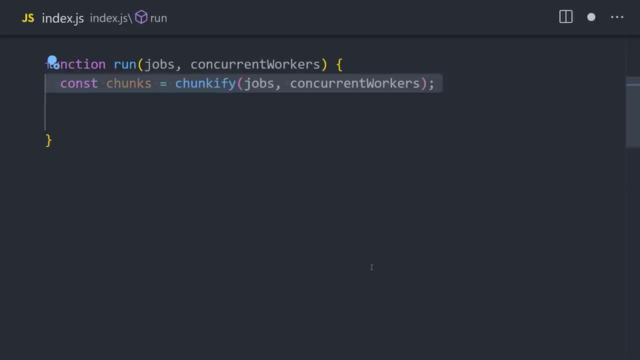 it into two parts, so that way each one of our workers is doing roughly the same amount of work. Like if we have 100 jobs and 4 CPU cores, each worker would get 25 jobs From there. we can loop over each one of those chunks and then instantiate a new worker by pointing. 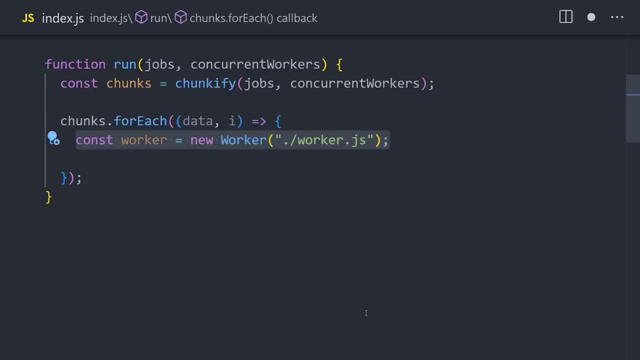 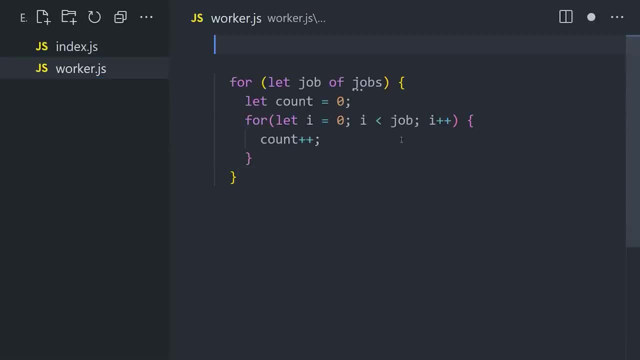 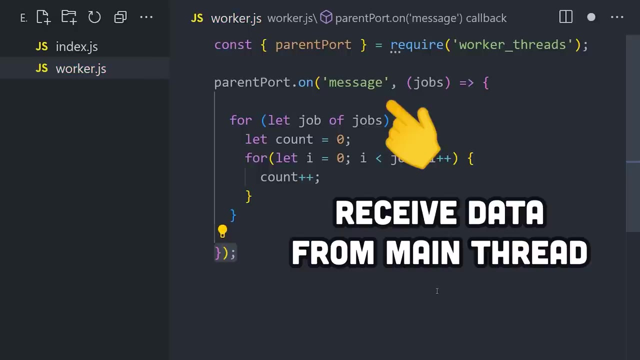 and see how we can receive that message. By importing the parent port from the worker threads module, we can receive that message from the main thread. The message will contain the data we passed in from the main thread and allows us to execute a callback function. 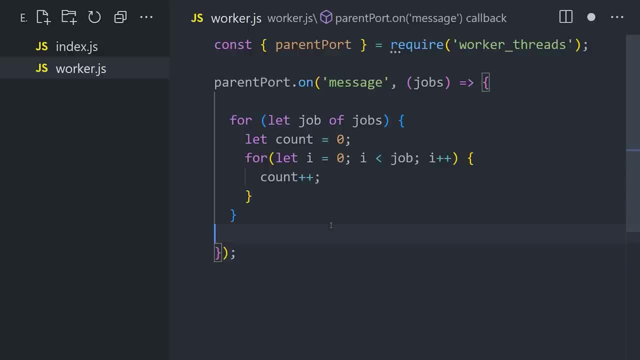 to process that data on a completely separate thread, which is automatically allocated by your machine. Now, finally, when the work is done, you'll need to notify the main thread, which is accomplished by calling postMessage. With this method, you can pass data back to. 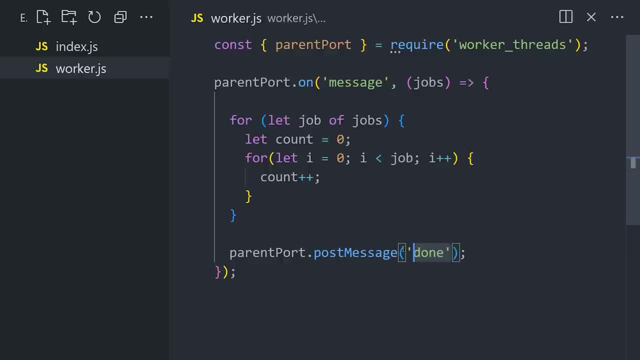 the main thread or, in this case, we'll just simply tell it that we're done, Although you could just do processexit here if you don't want to pass any data Now. the final step is to listen to messages on the main thread from the workers. 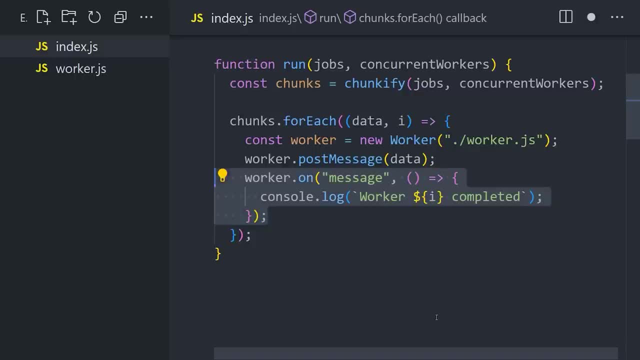 For each worker. we'll set up a listener for the message, at which point we'll know the worker has completed. In real life, though, you'd likely want to collect the data from the worker and do something with it. on the main thread, You might also be wondering if threads can share data while 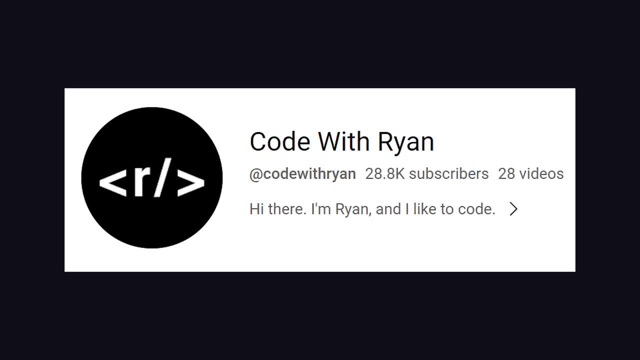 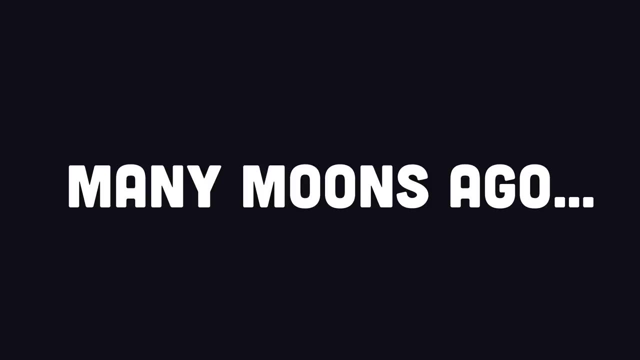 they run and the answer is yes. There's a channel called Code with Ryan that has a great video about this called Nodejs is a serious thing now, but I'm not going to get into it in this video because a long time ago I tried to synchronize data across threads in Python and I ended up with 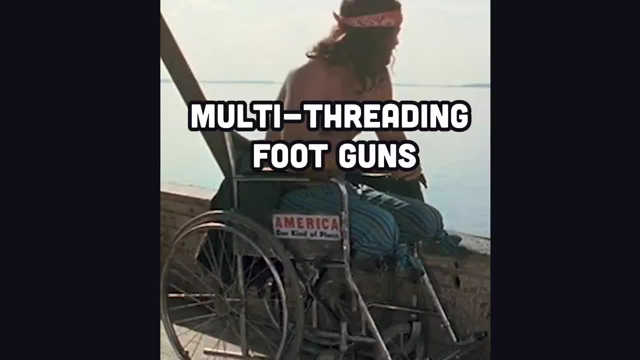 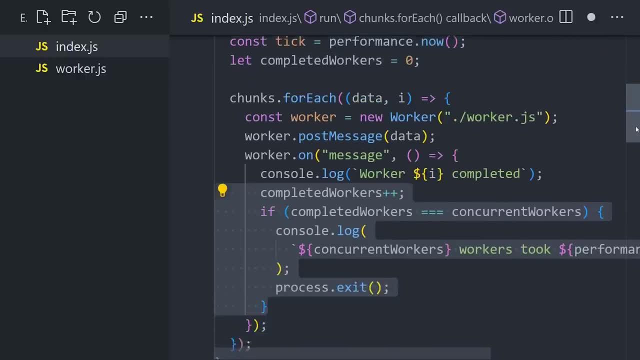 so many race conditions that the doctors had to amputate my leg. But now it's time to find out if this code results in any actual kind of performance gains. The last thing I'll do here is use the Nodejs performance module to measure the amount of time it takes for all the workers. 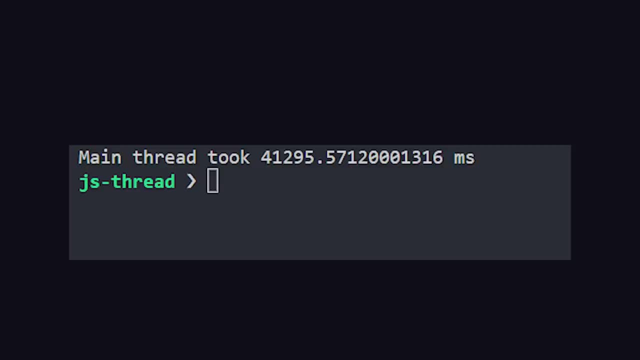 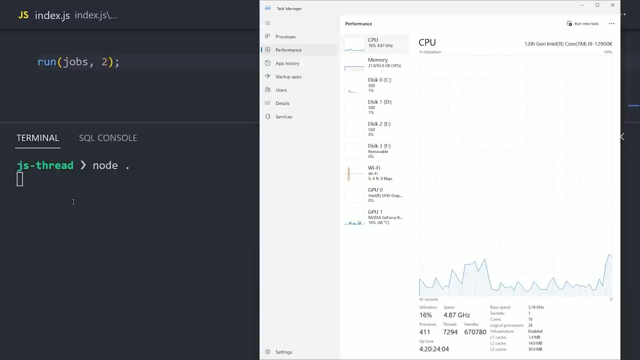 to complete and now we're ready to fire up the V8 engine. Remember, the first run on the main thread took 44 seconds, so now let's go ahead and run two workers in parallel. Currently, my CPU usage is at about 5%, but that should change. after we run this code, We see a definite 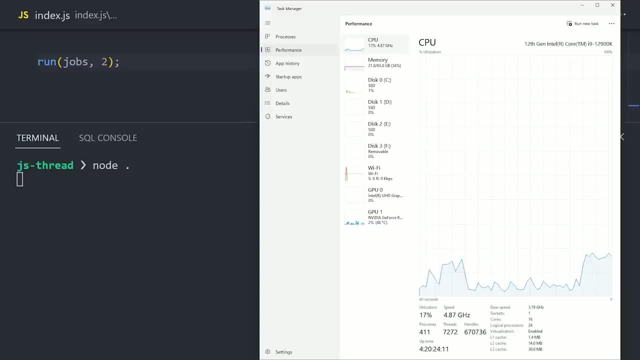 change in the code and now we're ready to fire up the V8 engine. We see an increase in utilization up to about 15%, and then the total execution time was about 20 seconds, roughly twice as fast as the initial run on the main thread. And that's exactly what. 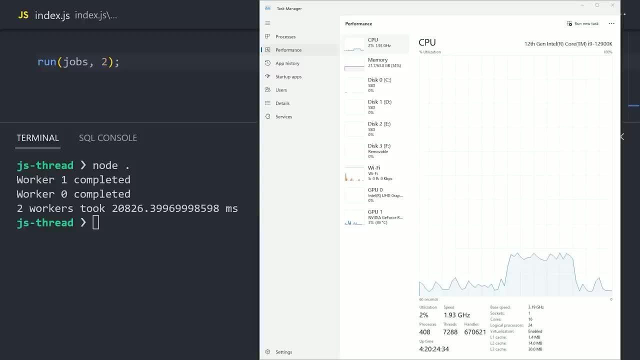 we would expect, because we're now using two threads instead of one. But now let's find out what happens when we give it some more juice. with four workers, As expected, CPU usage goes up to about 30% and the execution time is once again cut in half to about 10 seconds. Let's 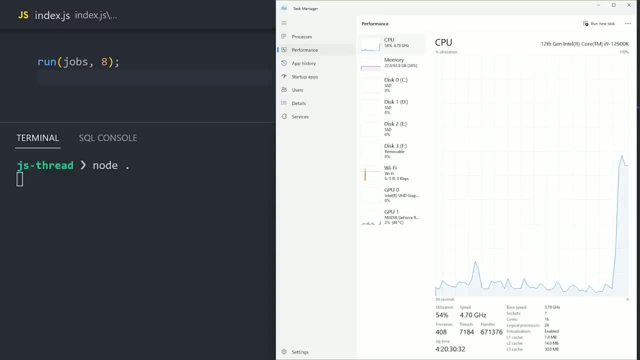 go ahead and double it again to eight workers Now. this time CPU usage goes above 50%, because that's half of our available threads and total execution time is about 10 seconds. The total execution time goes down to 6.2 seconds, a definite increase. but we're now starting to. 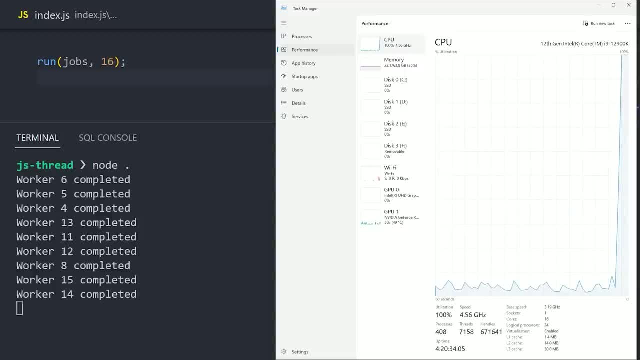 get some diminishing returns. Now, finally, let's go ahead and give it everything we've got with 16 workers. This time, the CPU goes to 100% utilization and total execution time comes down to 4.7 seconds, making it a total of 10 times faster than the initial run on the main thread. 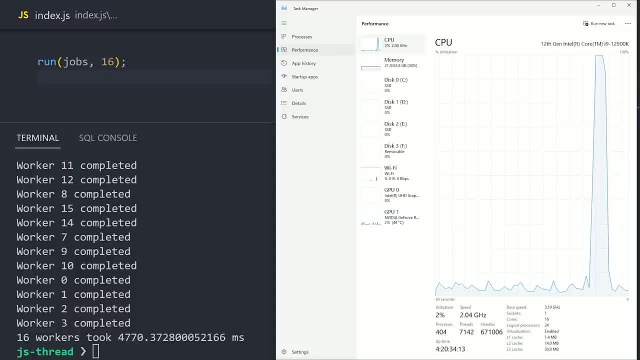 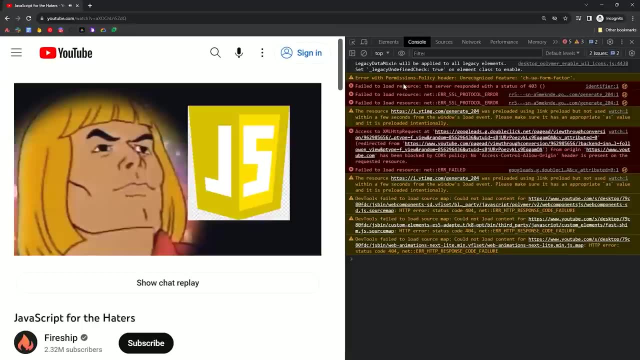 Now we could continue to add more workers, like say 100, but there will no longer be any increase in performance because there's no available CPU cores to use those threads. Everything on the main thread is still the same as it was in the initial run on the main thread. So let's. 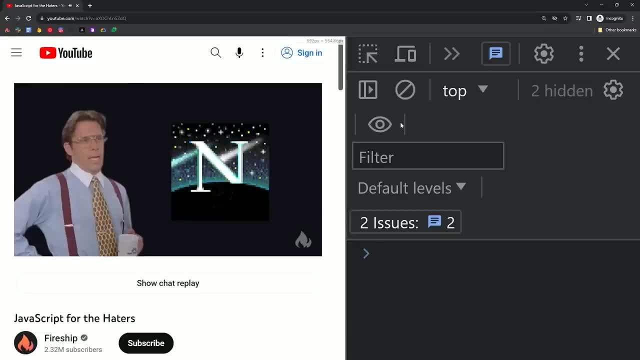 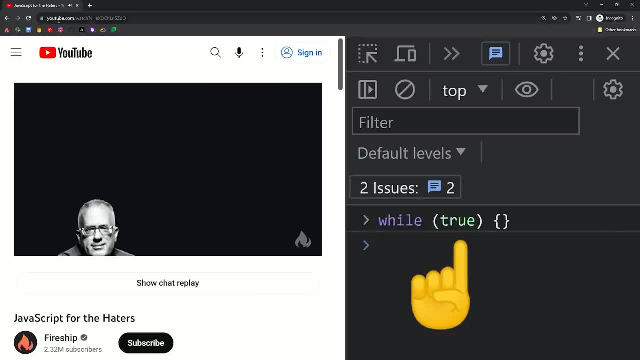 go ahead and open up your browser dev tools Inside the console, create a while loop with a condition of true and then, inside the brackets, just go ahead and do nothing. I'll go ahead and give you a moment to do that, because it's important to run this code while the video. 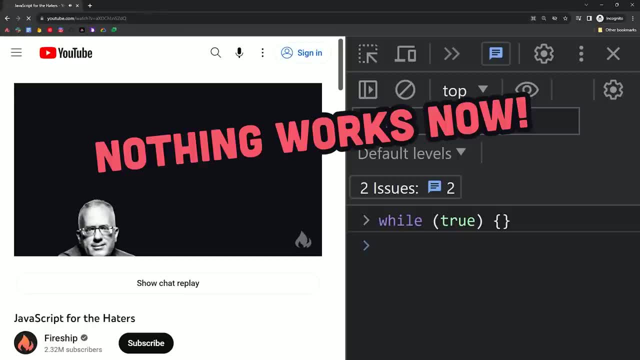 is playing. Remember, the browser is also single threaded, so when you run this code, it will lock up the main thread and the page should become unresponsive, And that means you'll be stuck on this video, allowing me to achieve infinite watch time. I can now tell you anything.